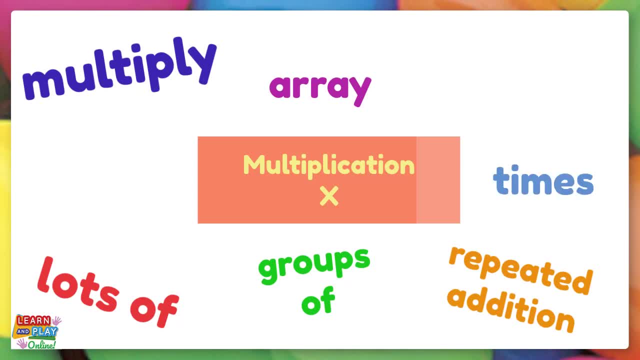 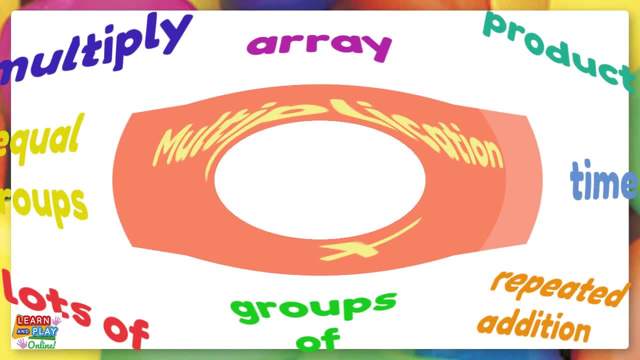 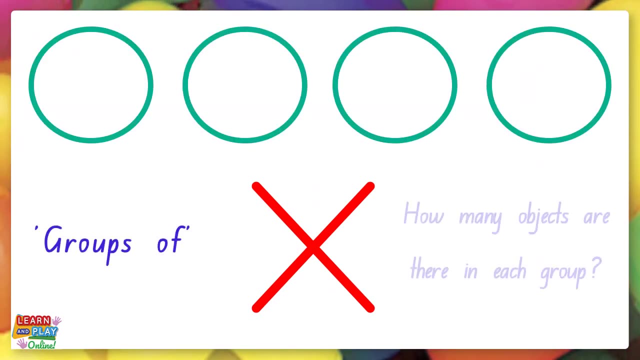 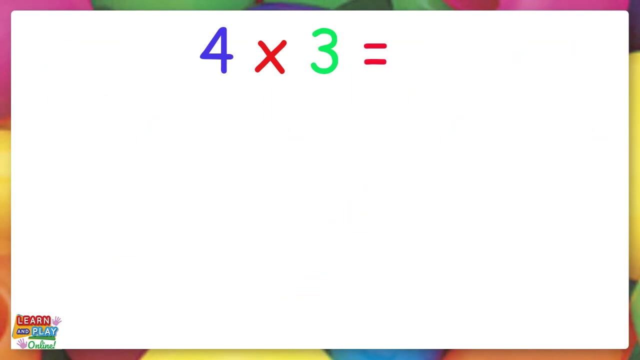 addition array times: product equal groups. In this video, we will be showing you how to solve multiplication problems using groups of and how many objects there are in each group. Let's start with a question that says four times three: What is multiplication? 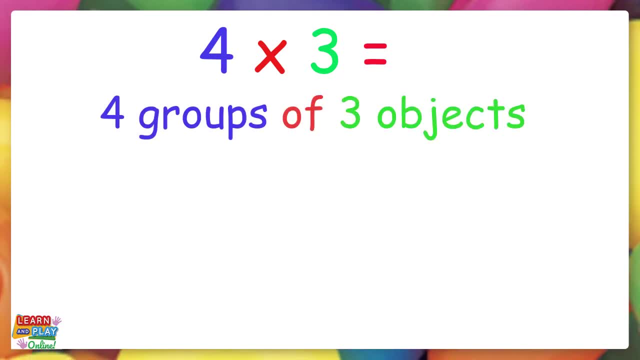 Multiplication is finding the total of equal-sized groups. Multiplication is finding the total of equal-sized groups. Multiplication is finding the total of equal-sized groups. We need to make four groups of three objects. Let's make four groups first: One, two, three, four. 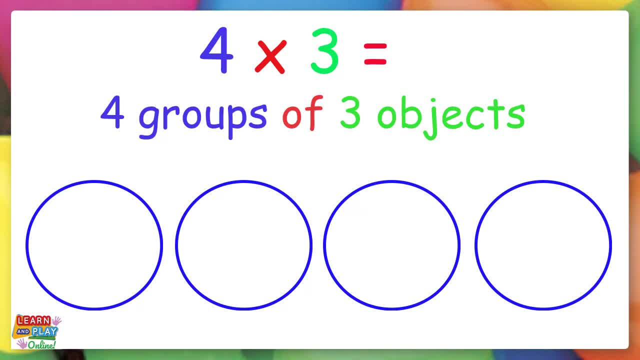 Now let's use stars as our objects, and we're going to put three stars in each group. Now we have made four groups of three stars in each group. How many stars do we have all together? Twelve stars, That's right. So the answer to four times three equals twelve. 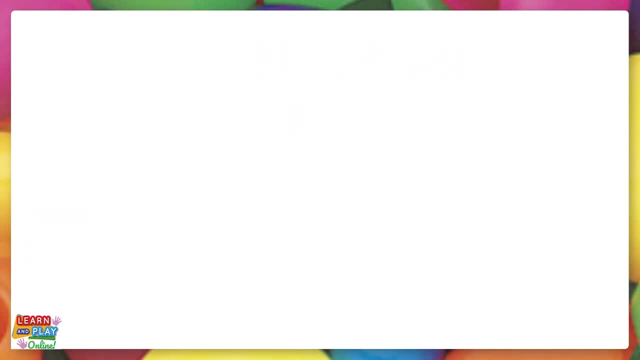 Now let's swap the numbers over and have the question as three times four. What do you think the answer will be? To find the answer to this question, we need to make three groups of four objects. Let's make three groups of four objects. 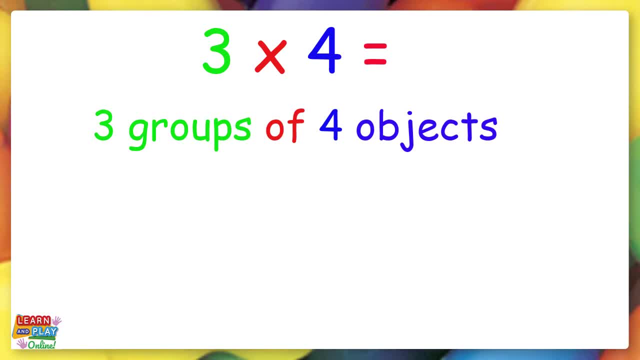 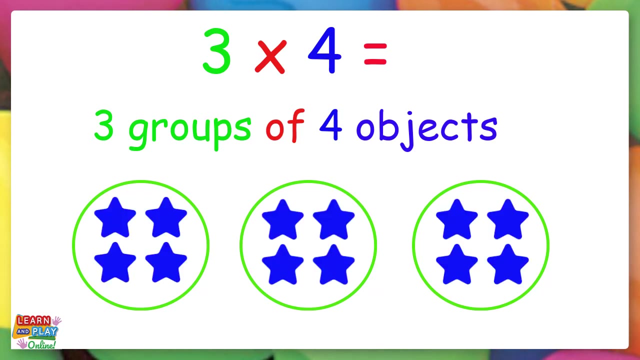 Let's make three groups of four objects. How many stars do we have altogether? Twelve stars, three groups: first, one, two, three. now we need to put four stars in each of the three groups. now have a look at how many stars we have all together. 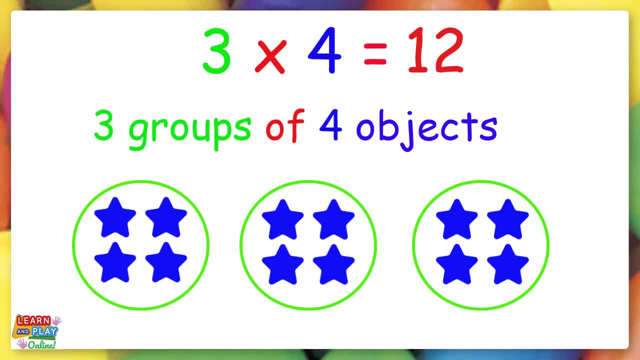 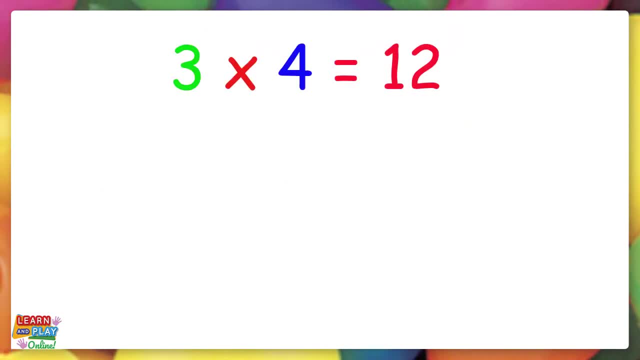 twelve stars. that's right. so the answer to three times four is also twelve. as you can see, three times four equals twelve and four times three also equal twelve. this is called commutative property, which means that we will get the same answer even if we swap the numbers over. let's try another question. this time our question is three times six.